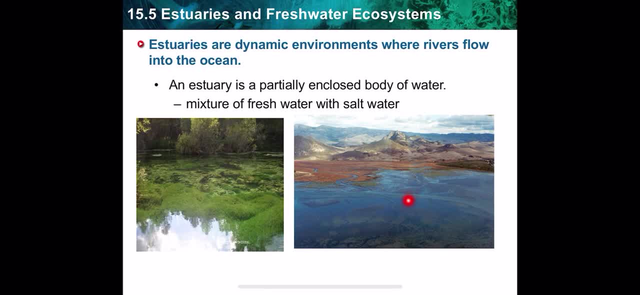 While when the ocean floods, The salty water will be more than the fresh water. Also, when rivers flow into ocean, the rivers will carry a lot of nutrients and sediments, which help the growing of many types of plants and algae. As you see in this picture, there are many types of plants and algae. 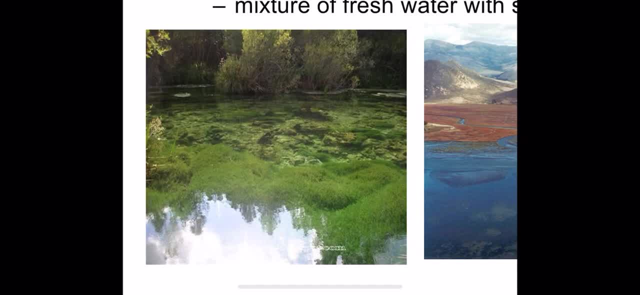 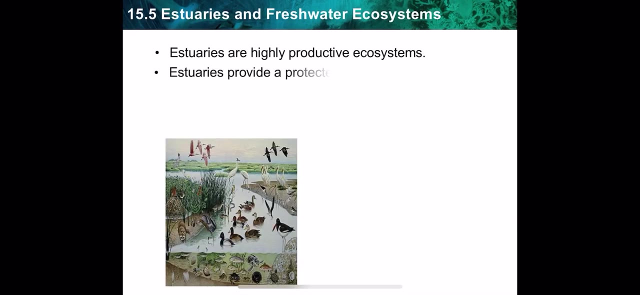 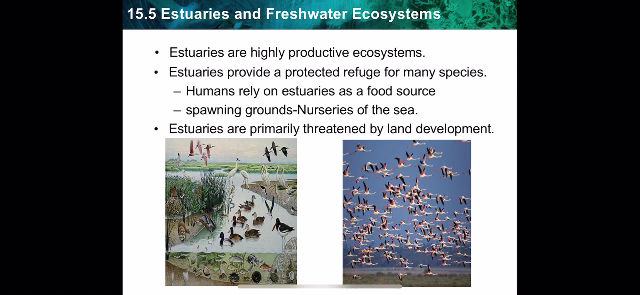 So this area is considered like A high productive area. A high productive area because of the nutrients, plants and the existence of algae. So what's the importance of estuaries? Number one: it's a highly productive area. 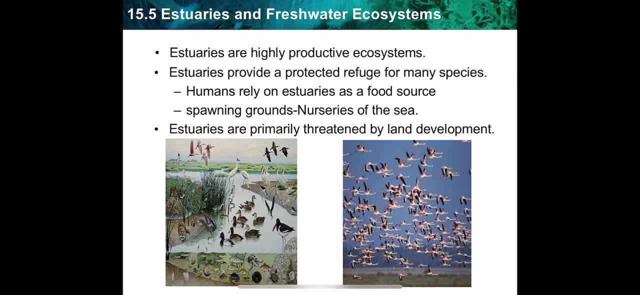 And also the water. there is not flowing water And there is no wave action. So the water there is constant And calm water Which helps the laying down or the laying of eggs. This will help many birds and fishes to lay their eggs there. 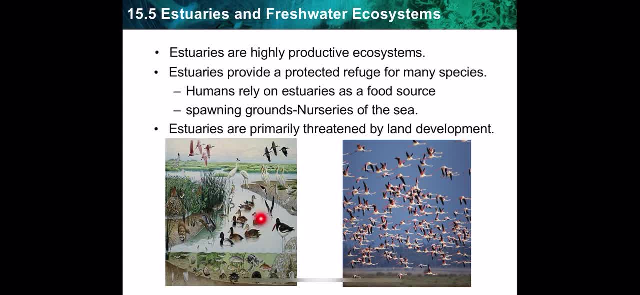 So it's considered like nurseries of the sea, Or an area for Or a spawning ground. Also, estuaries are important due to its high productivity and biodiversity, So the human will rely on, Will rely on the estuaries as a source of food. 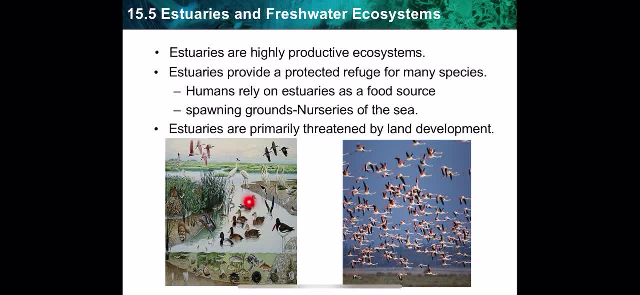 We can get many types of shrimps or fishes from estuaries. The existence of estuaries also will help the neighboring coastal areas from floods Because, as you know, the estuary like any other wetland, it can absorb water and carry. 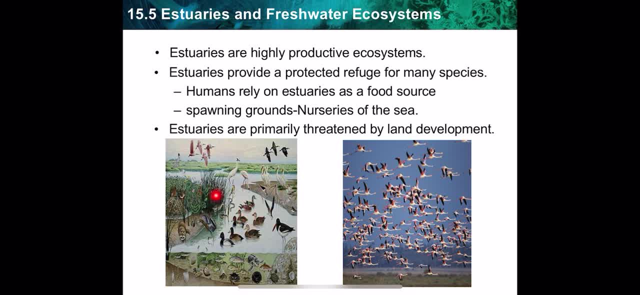 It can carry water to protect the neighboring areas from floods And, as you see in this picture, many birds can migrate also to estuaries Because it's a very rich and productive area where they can find fish to eat and plants And very good spawning area.